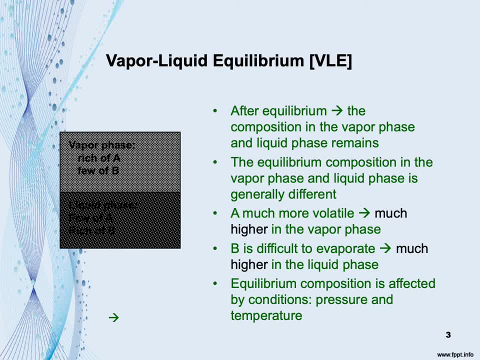 phase would be rich in a component a and just very few left in b and in the bottom phase of our sketch. this liquid phase b is difficult to offer evaporate so b will remain in the liquid phase with still a little bit of a. so a equilibrium composition is affected by conditions, the pressure. 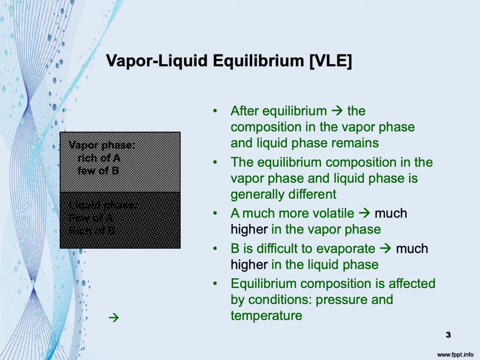 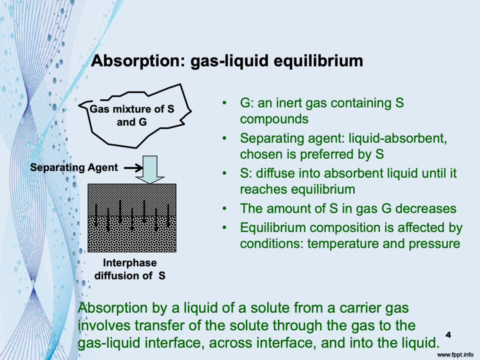 and temperature. also the composition, of course, of the those components. another example of application of separation processes is absorption. absorption is different with distillation, where absorption is actually gas liquid equilibrium. so in the first place we have a gas mixture comprised of, let's say, s, s is uh and g. let's say g is an inert gas and s is the. 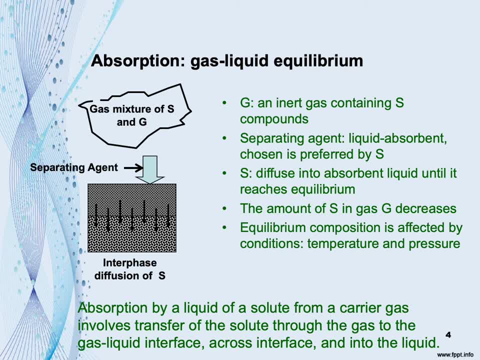 compound and we want to separate s from the g, so we add a separating agent. for this case it's a liquid absorbent, uh, which where the absorbent is uh much love to s, so it's chosen, preferred by us. so if we add the s into the mix, the gas mixture, and we have a very good mixture. s will diffuse into. 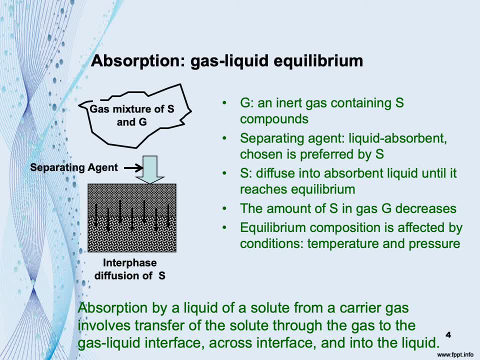 the ad servants liquid until it reach equilibrium, and then what we have in the end is the amount of s in the gas will decrease, while some of the s compound would be absorbed in the liquid separating agent. again, the composition is affected by temperature and pressure. yeah, so absorption is the liquid solute from the gas. carry grass. 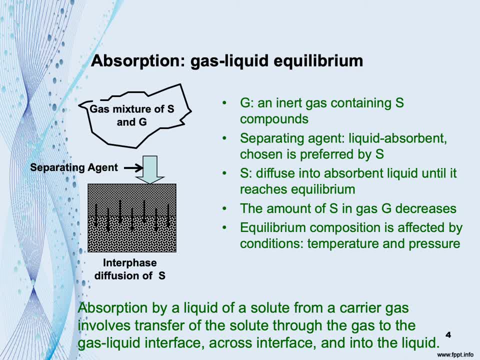 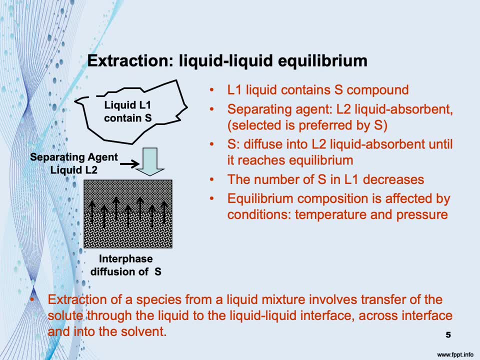 involves transfer of the solute through gas to the gas liquid interface, across interface and into the liquid. another example- this is going to be our last module- is extraction. extraction is a liquid liquid equilibrium. so we have a liquid one contained s, let's say, and we have liquid two also. 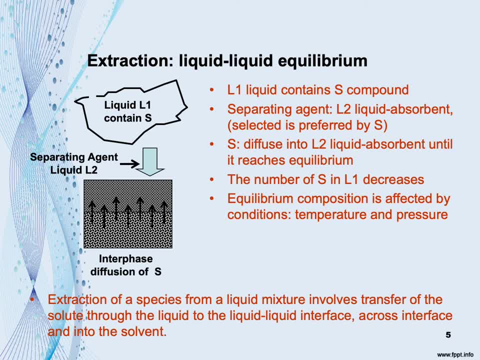 so um. so the separating agent is actually the liquid. to a liquid absorber, the, it is selected by a preferred bias. so the difference between absorption and absorption is the system started with a gas liquid, a system, but for um, in extraction it's contained liquid liquid system. 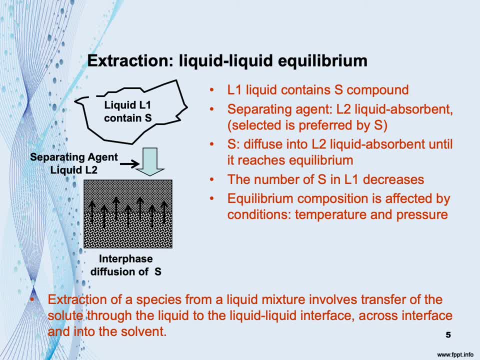 um. the equilibrium composition again is affected by condition so easily in extraction. we have uh two phase and in the end there would be uh an extract. an extract is uh the liquid that have contained more uh as compound that we want in the end and the remaining uh solution is called. 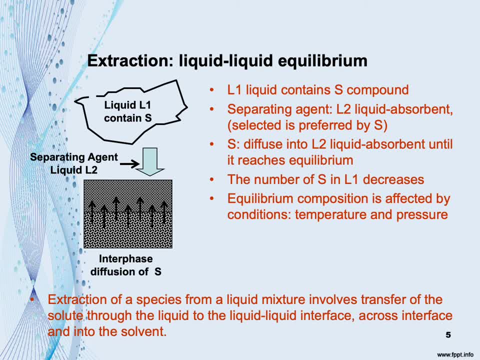 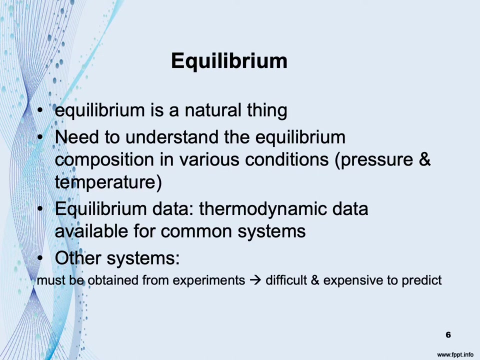 raffinate. raffinate is the uh, the, the remaining solution that still has a little bit of as compound. so extraction is spacious. from a liquid mixture. uh involves transfer of the solute through the liquid to the liquid liquid interface, across interface and into the solvent based on the uh- previous explanation. so 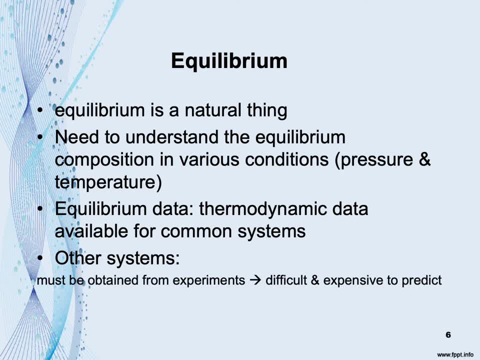 equilibrium is really natural things. this is that the the god give us, give it to us. so, uh, it's a function of temperature pressure and we need to understand equilibrium composition in various conditions. and equilibrium data is actually thermodynamic data and over the years- since 1940s, 1950s, so- scientists have gathered a lot of equilibrium data, so we have 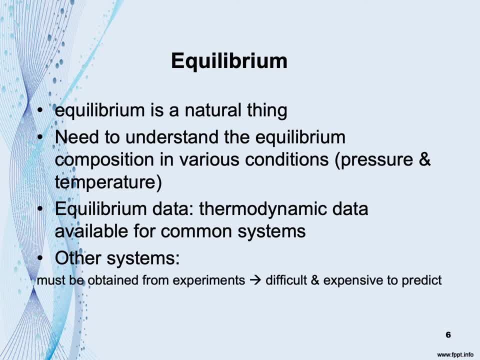 very uh vast uh terminic data available for common system. however, for other systems, that is quite new. uh, we need to uh make an experiment uh to uh to obtain the equilibrium data. so, uh, if we have other system that hasn't been um where the terminic not has been, uh, 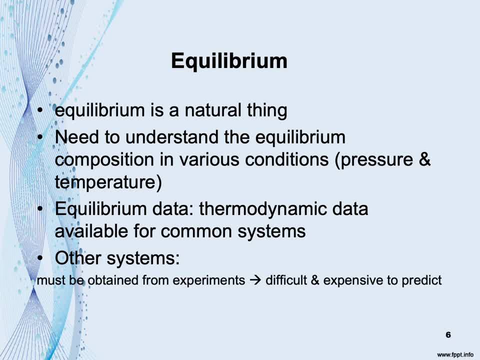 available. so we have to obtain from the experiments and it is difficult to uh to to do and also it's expensive to predict. okay,